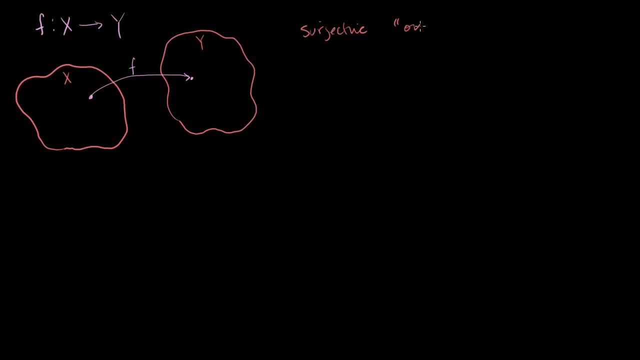 And sometimes this is called onto And a function is surjective or onto if for every element in your codomain. So let me write it this way: If for every, let's say, y, That is a member of my codomain. 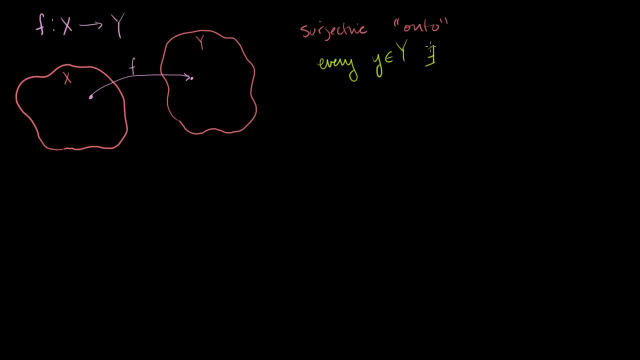 There exists. there exists- that's the little shorthand notation for exists- There exists at least one, at least one, at least one x that's a member of x. such that- and I could write such that, like that, Actually, let me just write the word out- such that, such. 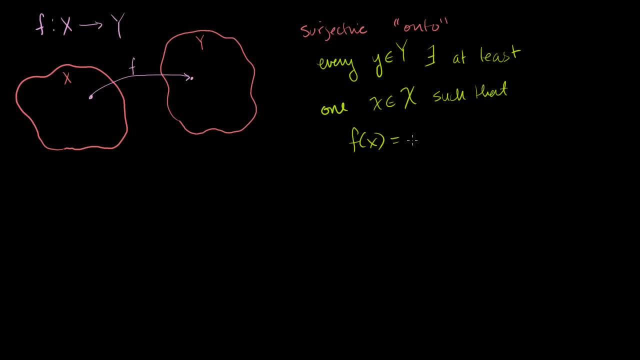 that f of x, f of x, is equal to y. So it's essentially saying: look, you can pick any y here, and every y here is being mapped to by at least one of the x's over here. So, for example- actually let me draw a simpler- 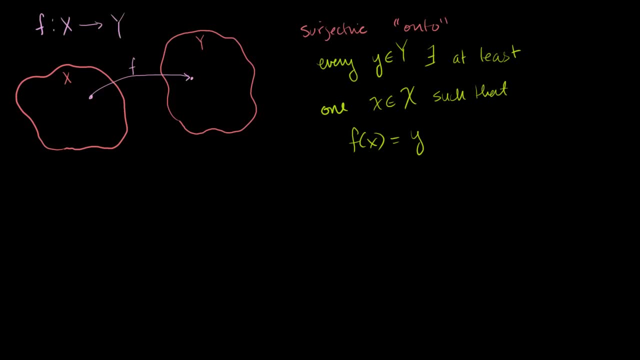 example, instead of drawing these blurbs, Let's say that I have a set y that literally looks like this. Let's say that a set y- I'll draw it very- and let's say it has four elements. It has the elements. 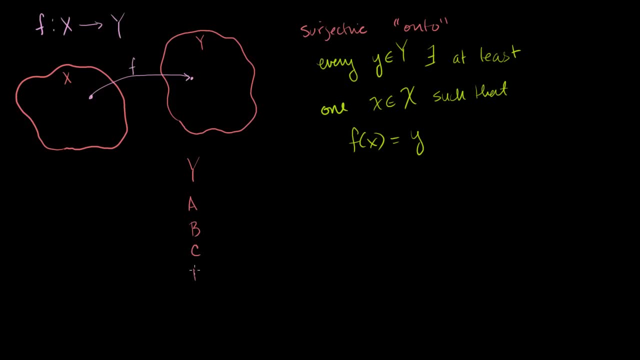 A, b, c and d. This is my set y, right there. And let's say my set x looks like that And let's say it has the elements- I don't know- 1,, 2,, 3, and 4.. 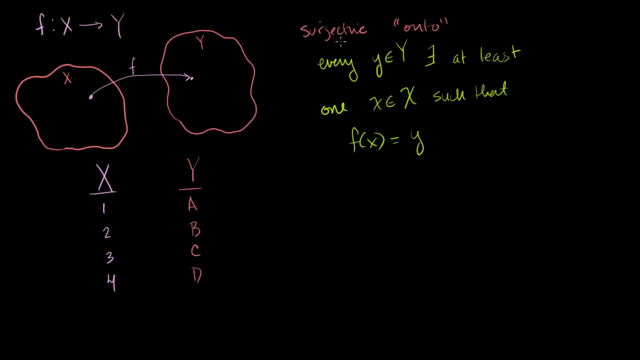 Now, in order for my function f to be surjective or onto, it means that every one of these guys have to be able to be mapped to. So what does that mean? So, if every one of these guys? let me just draw some examples. 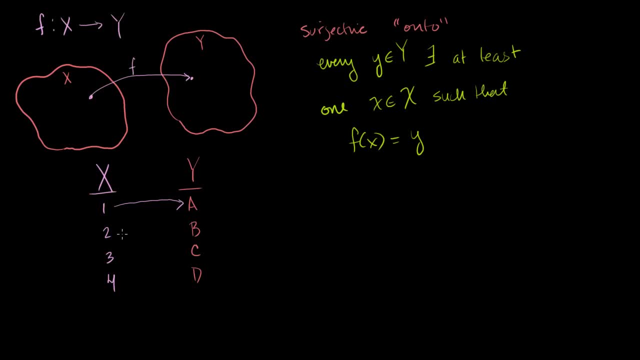 Let's say that this guy maps to that. Let's say that this guy maps to that. Let's say that this guy maps to that, And let's say, let me draw a fifth one right here. Let's say that both of these guys right here map to d. 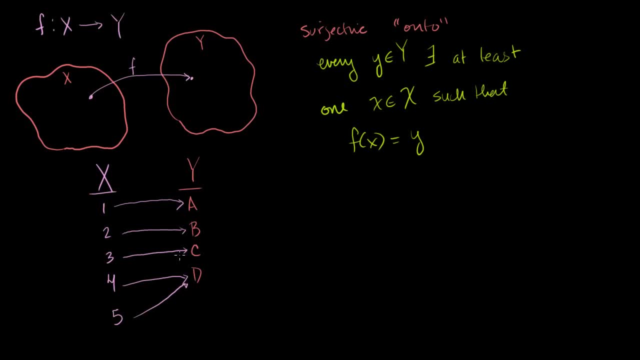 So f of 4 is d and f of 5 is d. This is an example of a surjective function. So these are the mappings of f right here. This function right here is on, Is onto or surjective. Why is that? 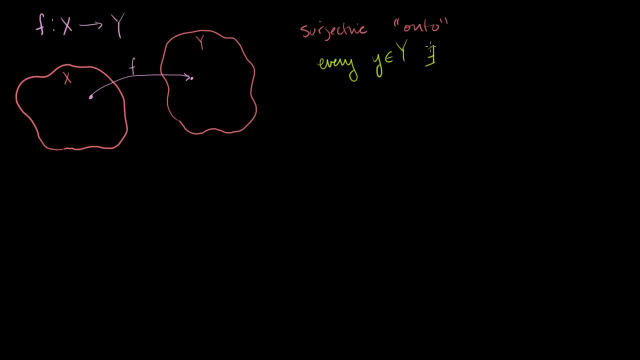 There exists. there exists- that's the little shorthand notation for exists- There exists at least one, at least one, at least one x that's a member of x. such that- and I could write such that, like that, Actually, let me just write the word out- such that, such. 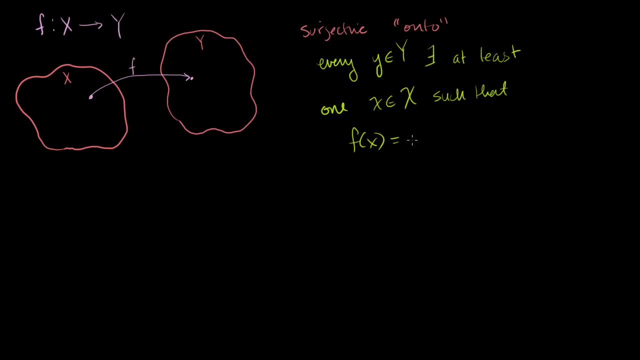 that f of x, f of x, is equal to y. So it's essentially saying: look, you can pick any y here, and every y here is being mapped to by at least one of the x's over here. So, for example- actually let me draw a simpler example. 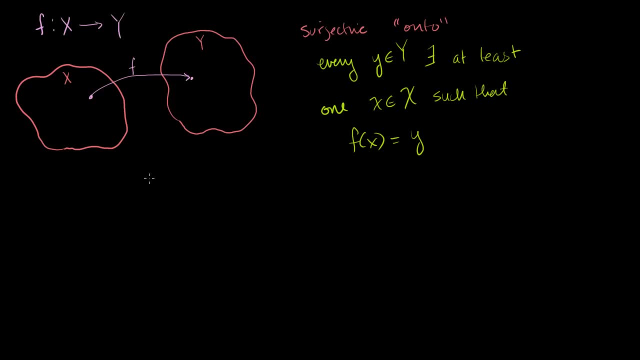 Instead of drawing these blurbs, let's say that I have a set y that literally looks like this. Let's say that a set y, I'll draw it very. and let's say it has four elements. It has the elements A y, z. 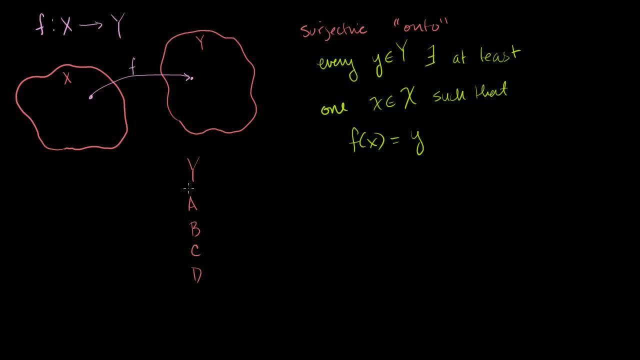 b, c and d. This is my set y, right there. And let's say my set x looks like that, And let's say it has the elements- I don't know- 1,, 2,, 3, and 4.. 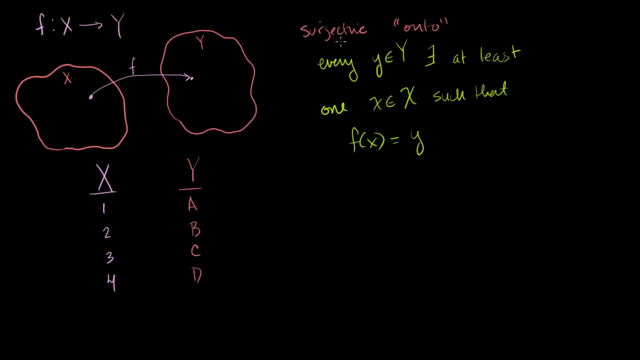 Now, in order for my function f to be surjective or onto, it means that every one of these guys have to be able to be mapped to. So what does that mean? So, if every one of these guys? let me just draw some examples. 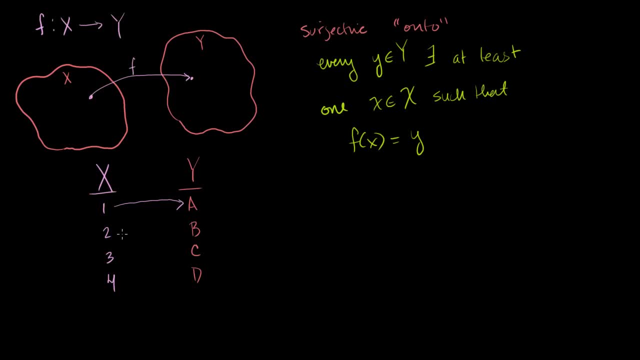 Let's say that this guy maps to that. Let's say that this guy maps to that. Let's say that this guy maps to that, And let's say, let me draw a fifth one right here. Let's say that both of these guys right here map to d. 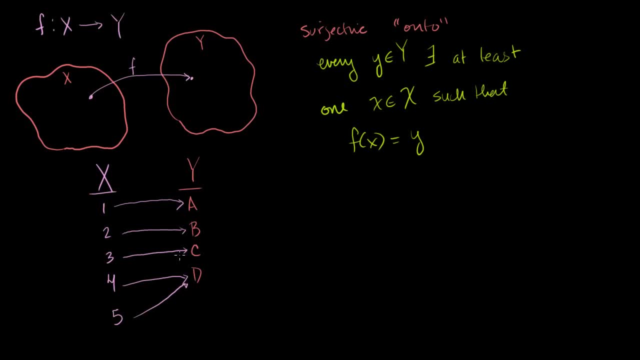 So f of 4 is d and f of 5 is d. This is an example of a surjective function. So these are the mappings of f right here. This function right here is on, Is onto or surjective. Why is that? 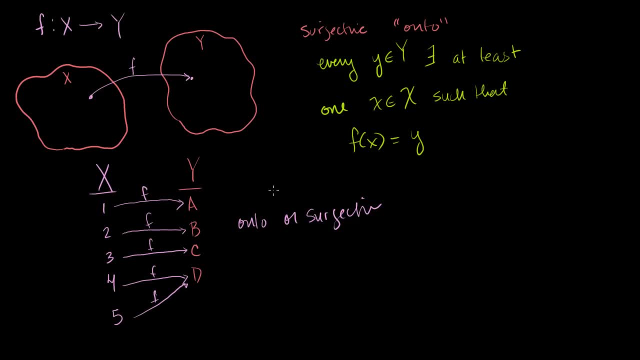 Because every element here is being mapped to. Now let me give you an example of a function that is not surjective. Let me add some more elements to y. Let's say y has another element here called e. Now, all of a sudden, this is not surjective. 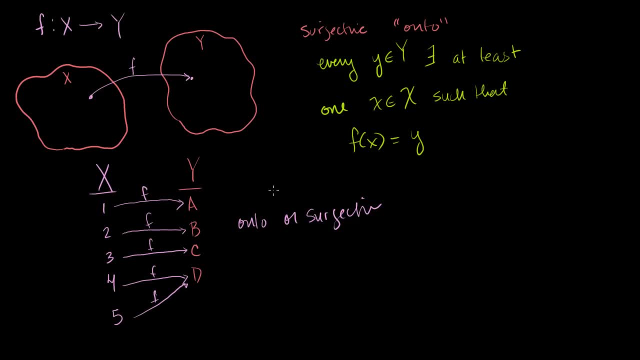 Because every element here is being mapped to. Now let me give you an example of a function that is not surjective. Let me add some more elements to y. Let's say y has another element here called e. Now, all of a sudden, this is not surjective. 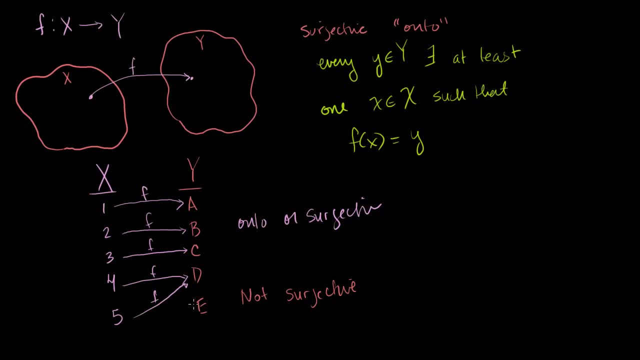 And why is that? Because there's some element in y That is not being mapped to. So if I tell you that f is a surjective function, it means that if you take essentially, if you map all of these values, everything here, 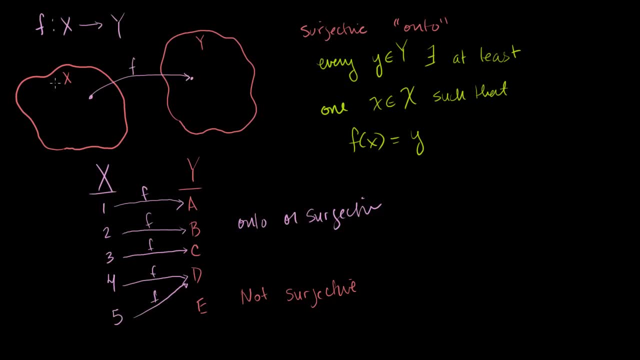 is being mapped to by at least one element here, So you could have it. you know, everything could be kind of a one-to-one mapping And I'll define that a little bit better in the future, So it could just be like that and like that. 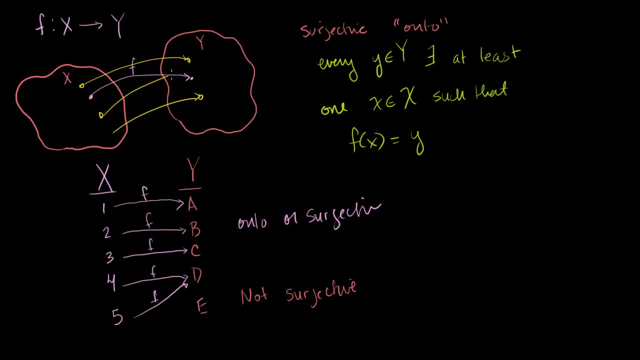 And you could even have it's at least one. So you could even have two things in here mapping to one thing in here, But the main requirement is that everything here does get mapped to. Another way to think about it is that if you take the image, 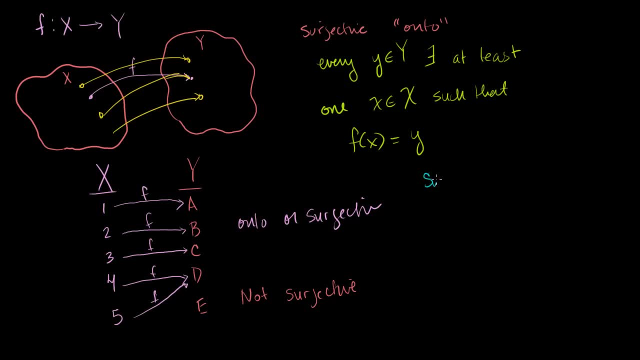 so a surjective function. let me write this here. Let me write it this way. So if I say that f is surjective or onto- these are equivalent terms- that means that the image, the image of f- remember, the image was all of the values. 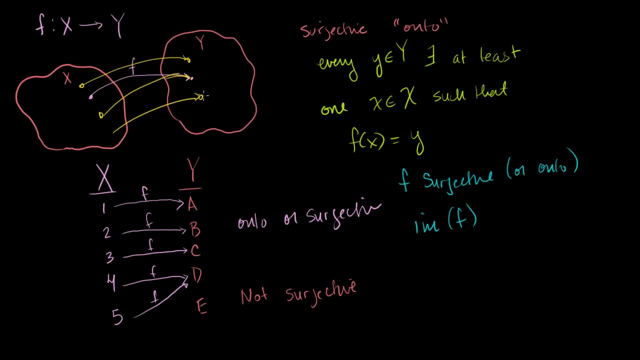 that f actually maps to. So that means that the image of f is equal to y. Now we learned before that your image doesn't have to equal your codomain, But if you have a surjective or an onto function, your image is going to equal your codomain. 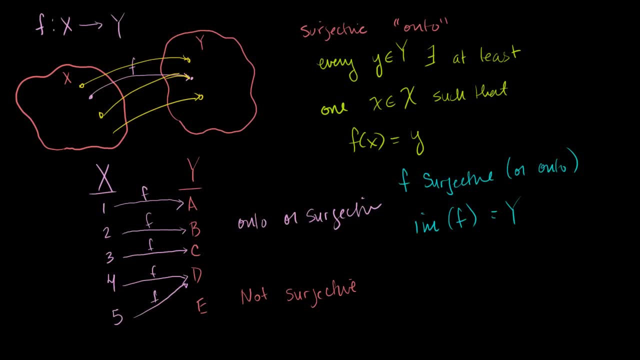 Everything in your codomain gets mapped to. And actually, another word for image is range. You could also say that your range, your range of f, is equal to y. Remember the difference, and I drew this distinction when we first talked about functions- the distinction between a. 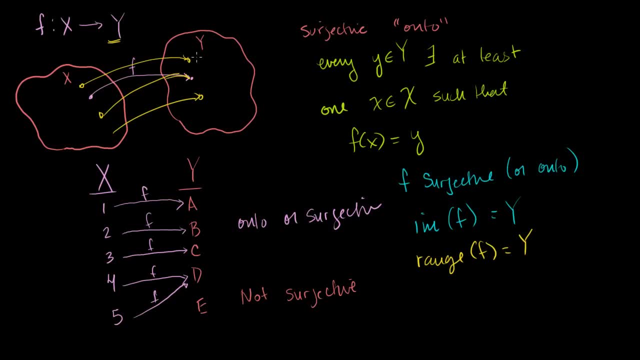 codomain and a range. a codomain is a set that you can map to. you don't have to map to everything. The range is a subset of your codomain. a range is a subset of codomain of your codomain that you actually do map to. 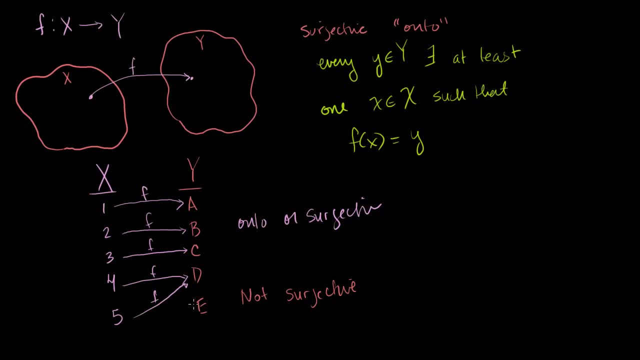 And why is that? Because there's some element in y That is not being mapped to. So if I tell you that f is a surjective function, it means that if you take essentially, if you map all of these values, everything here, 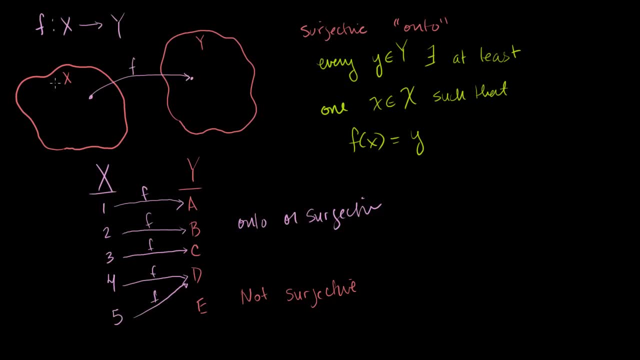 is being mapped to by at least one element here, So you could have it. you know, everything could be kind of a one-to-one mapping And I'll define that a little bit better in the future, So it could just be like that and like that. 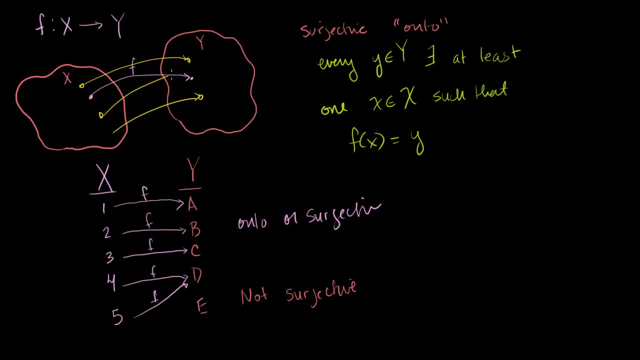 And you could even have it's at least one. So you could even have two things in here mapping to one thing in here, But the main requirement is that everything here does get mapped to. Another way to think about it is that if you take the image, 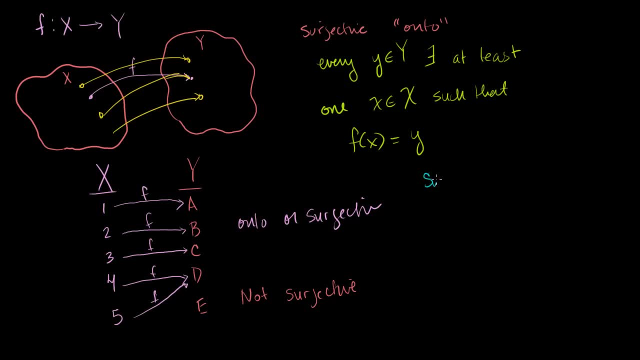 so a surjective function. let me write this here. Let me write it this way. So if I say that f is surjective or onto- these are equivalent terms- that means that the image, the image of f- Remember, the image was all of the values. 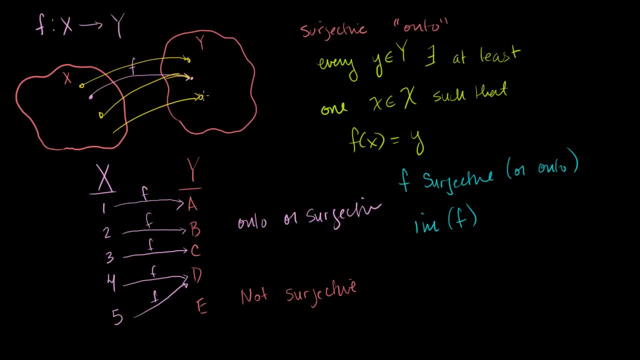 that f actually maps to. So that means that the image of f is equal to y is equal to y. Now we learned before you know your image doesn't have to equal your codomain, But if you have a surjective or an onto function, 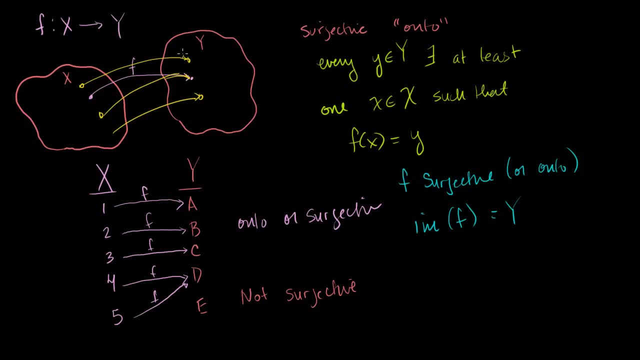 your image is going to equal your codomain. Everything in your codomain gets mapped to, And actually another word for image is range. You could also say that your range, your range of f, is equal to y. Remember the difference, and I drew this distinction when we 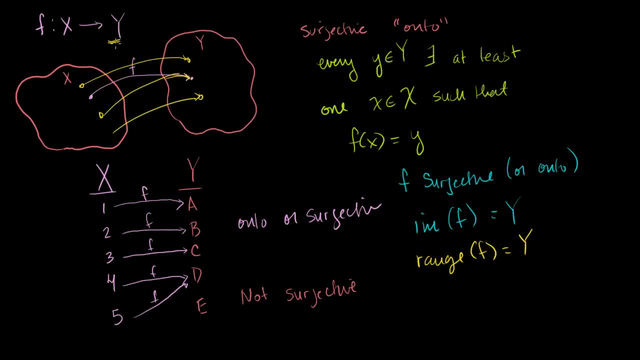 first talked about functions, the distinction between a codomain and a range. a codomain is a set that you can map to. you don't have to map to everything. The range is a subset of your codomain. a range is a subset. 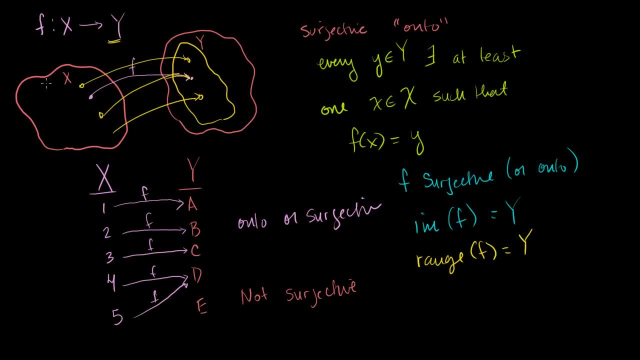 of codomain, of your codomain that you actually do map to, If you were to evaluate the function at all of these points. the point that you actually map to is your range, And that's also called your image, and we use the. 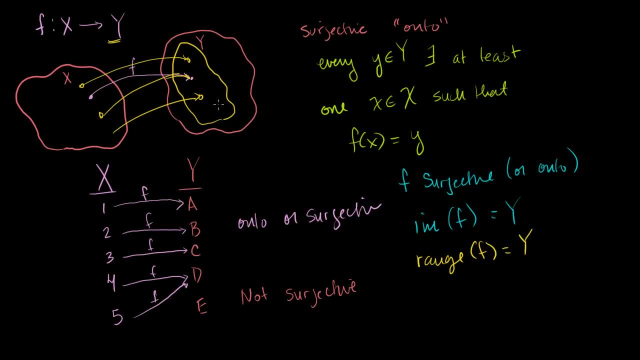 If you were to evaluate the function at all of these points. the point that you actually map to is your range, And that's also called your image and we use the image. The word image is used more in a linear algebra context, But if your image or your range is equal to your codomain, if 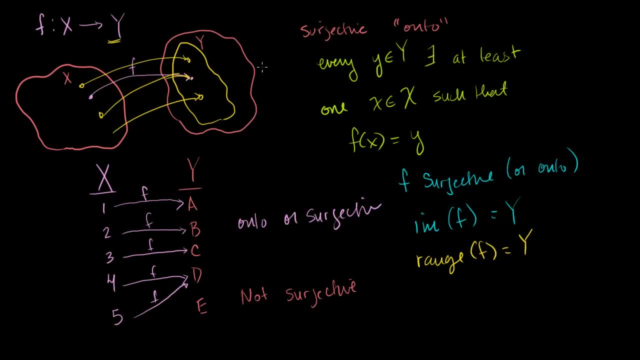 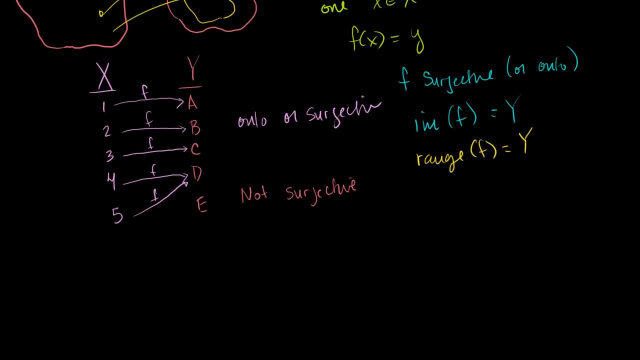 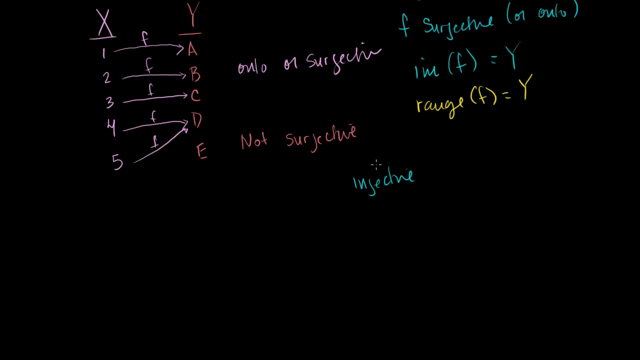 everything in your codomain does get mapped to, then you're dealing with a surjective function or an onto function. Now, the next term I want to introduce you to is the idea of an injective function: Injective, Injective, Injective function. 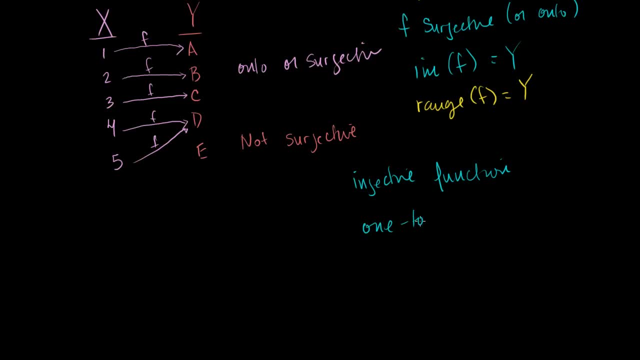 And this is sometimes called a one-to-one function. So let me draw my domain and codomain again. So let's say that that is my domain and this is my codomain. So this is x and this is y. If I say that f is injective or one-to-one, that implies that 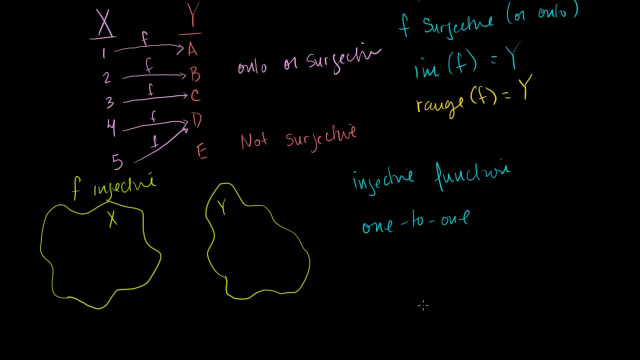 for every value that is mapped to. so let me write it this way: for every value that is mapped to. so let's say, I'll say it a couple of different ways. there is at most one x that maps to it. There is at most one x that maps to it. 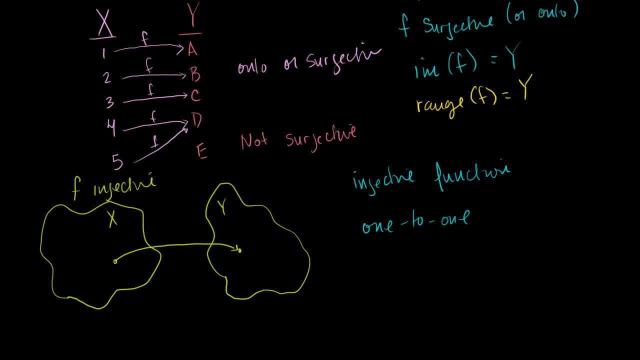 Or another way to say it is that for any y that's a member of y, let me write it this way- for any y that is a member of y, there is at most one, at most- let me write most in capital- at most one x, such that f of x is equal to y. 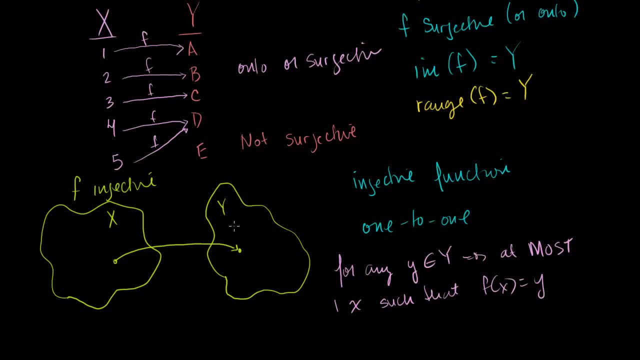 There might be no x's that map to it. So, for example, you could have a little member of y right here that just never gets mapped to. You know everyone else in y gets mapped to, but that guy never gets mapped to. 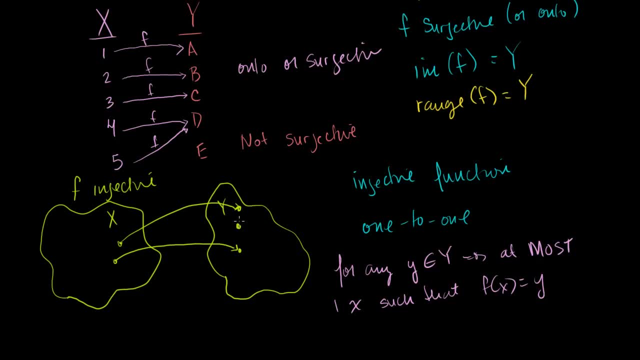 So this would be a case where we don't have a surjective function. this is not onto, because this guy is not. he's a member of the codomain, but he's not a member of the image or the range. He doesn't get mapped to. 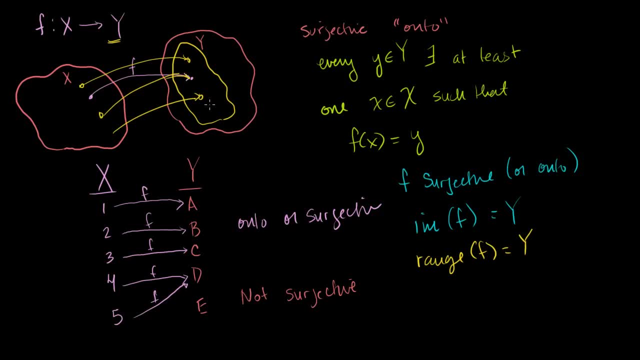 image. the word image is used more in a linear algebra context, but if your image or your range is equal to your codomain, if everything in your codomain does get mapped to, then you're dealing with a surjective function or an onto function. 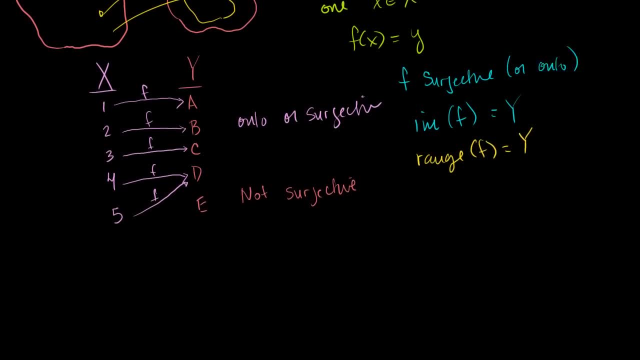 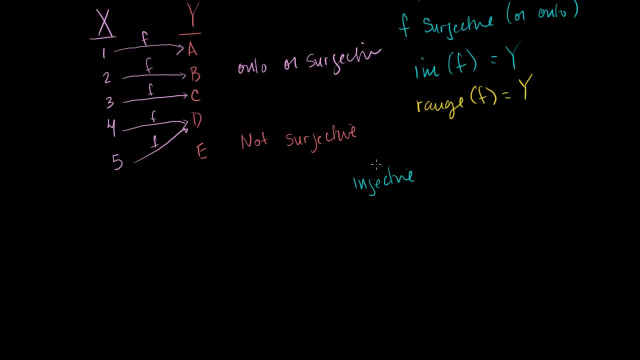 Now, the next term I want to introduce you to is the idea of an injective function, And this is sometimes called a one-to-one function. So let me draw my domain and codomain again. So let's say that that is my domain and this is my. 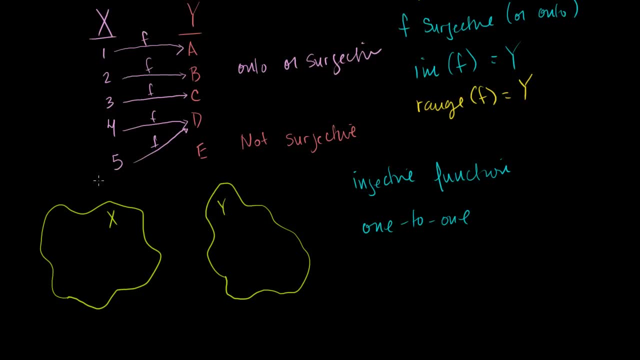 codomain, so this is x and this is y. If I say that f is injective or one-to-one, that implies that for every value that you have, you're going to have to keep is mapped to. so let me write it this way: for every value. 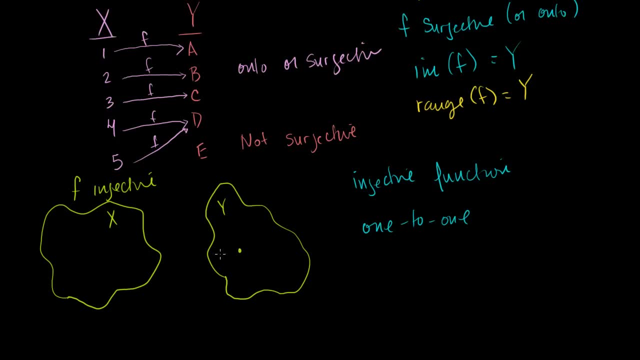 that is mapped to. so let's say- I'll say it a couple of different ways- there is at most one x that maps to it. Or another way to say it is that for any y that's a member of y, let me write it this way- for any y that is a member of, 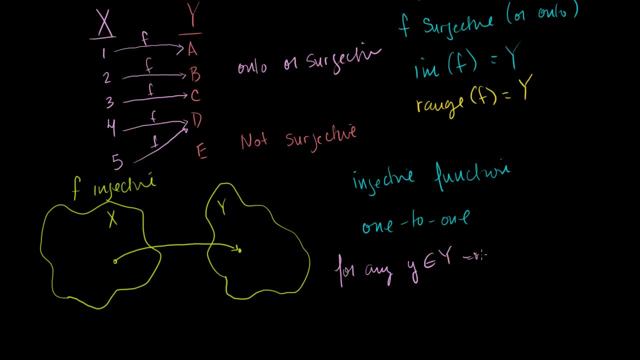 y, there is at most one x, such that f of x is equal to y. There might be no x's that map to it. So, for example, you could have a little member of y right here that just never gets mapped to. Everyone else in y gets mapped to, but that guy never gets. 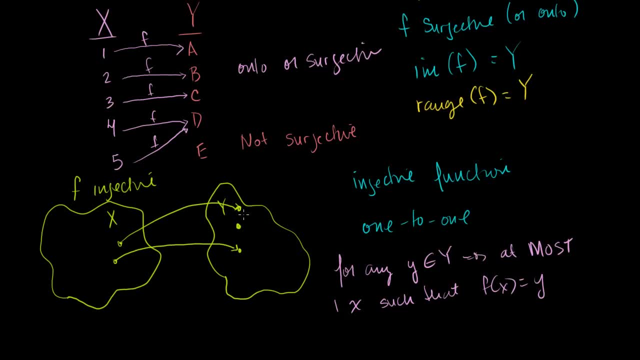 mapped to. So this would be a case where we don't have a surjection. This is an injective function. this is not onto, because this guy is not. he's a member of the codomain, but he's not a member of the image or the range. 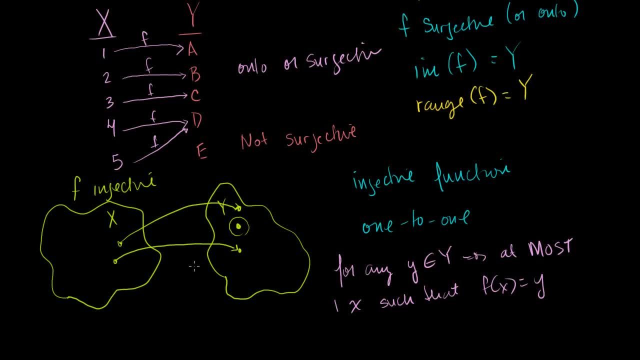 He doesn't get mapped to. But this would still be an injective function as long as every x gets mapped to a unique y. Now how can a function not be injective or one to one? And I think you get the idea when someone says one to one.